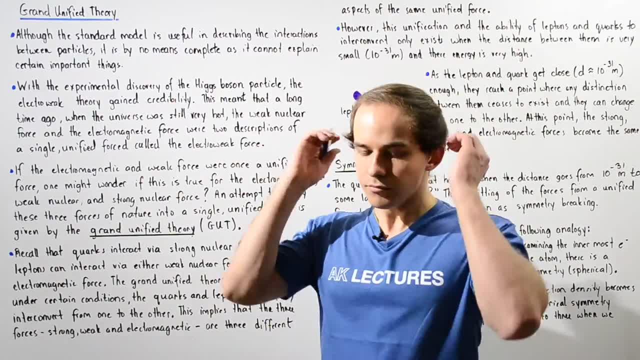 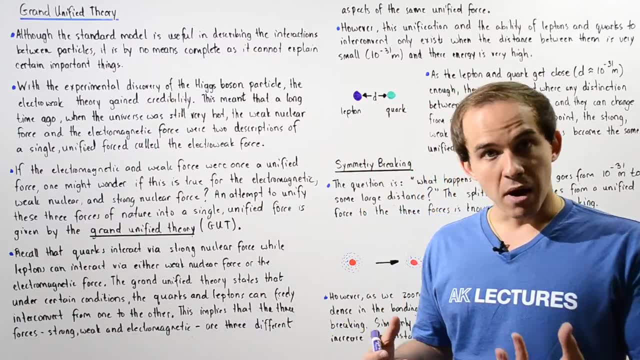 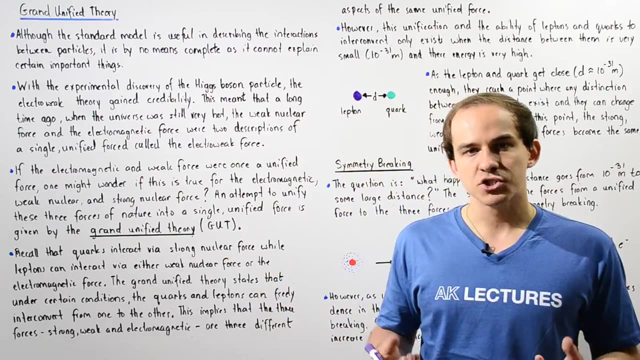 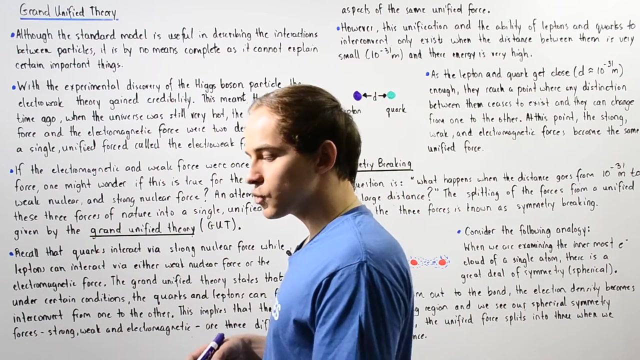 Grand Unified. In our previous discussion, we said that the theory or model that describes the way that particles interact with one another in particle physics is known as the standard model. Now, although the standard model can be very useful in helping us understand and describe the way that particles interact with one another, it is by no means a complete. 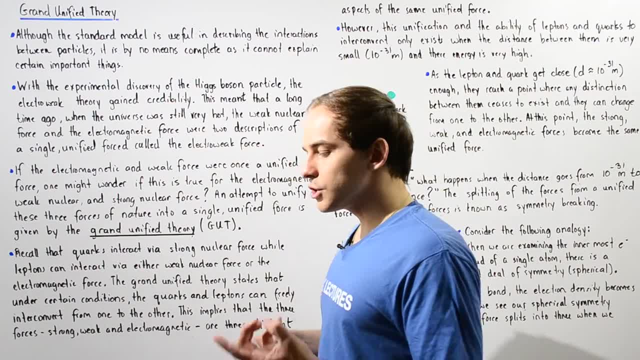 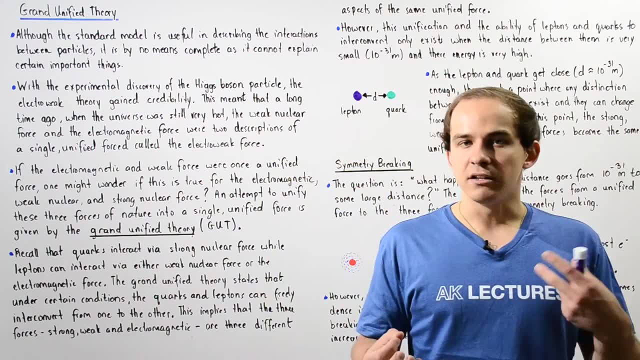 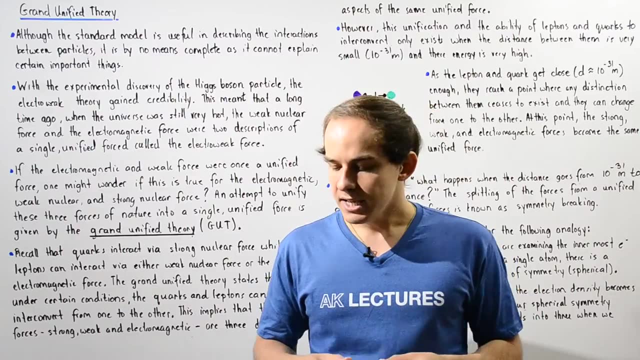 model because it cannot explain certain important things about nature. For example, it cannot explain why protons and electrons have the same magnitude or quantity of electric charge, but opposite in science. So with the discovery of the Higgs boson particle into the atmosphere, we can now understand that the Higgs boson particle is a particle. 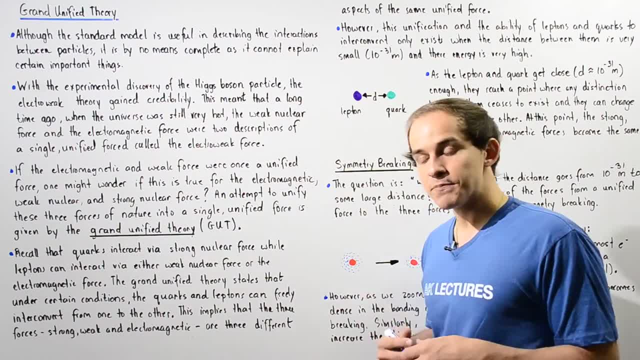 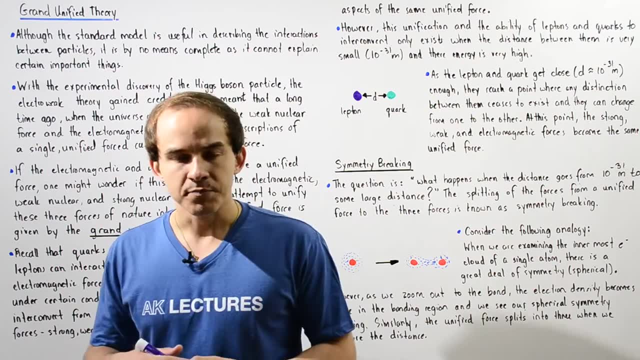 but opposite in science. So with the discovery of the Higgs boson particle into the atmosphere 2012,, with experimental evidence for this type of particle, we were basically able to confirm the electroweak theory. The electroweak theory is basically the theory that unifies the 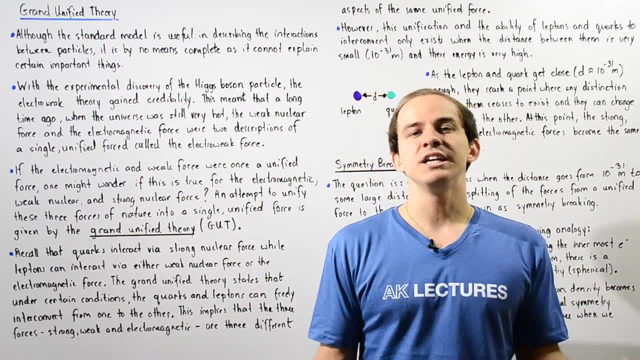 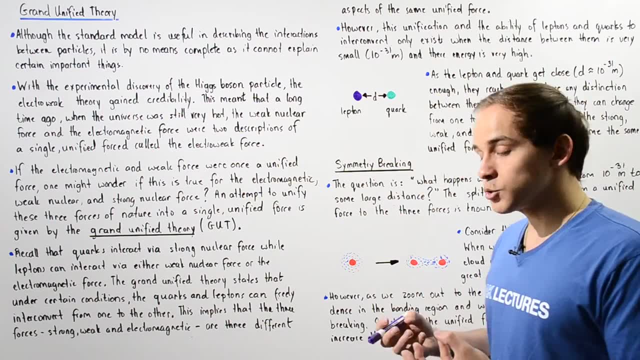 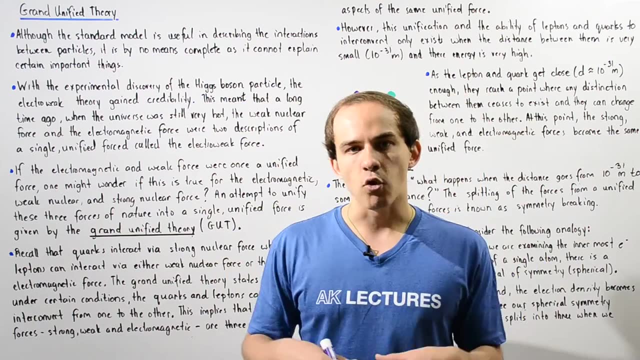 electromagnetic force and the weak nuclear force into a single force. So basically a very long time ago, when our universe was still very, very hot, these two forces, the electromagnetic force and our weak nuclear force, were basically a single force we call the electroweak force. 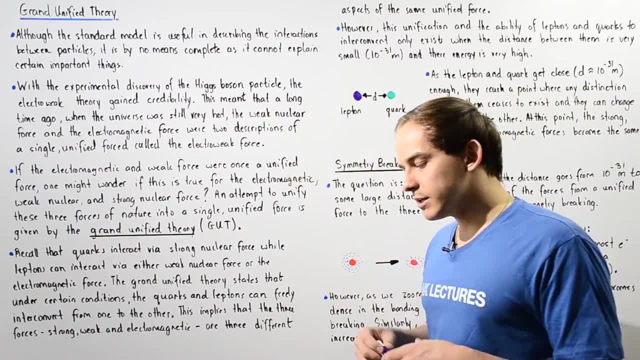 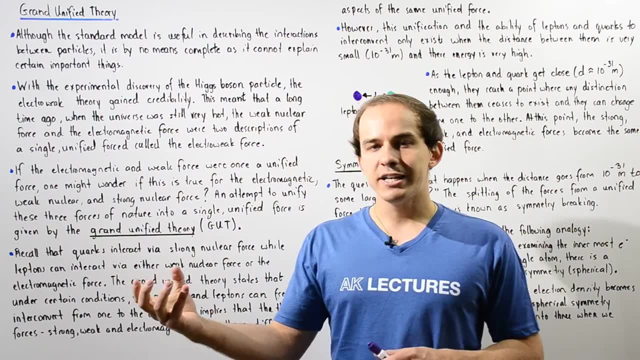 Now the question that theoretical physicists are trying to answer is if we can combine the electromagnetic force and our weak nuclear force into a simple physical form. what are the possibleiches and forms of energy that could absorb the electroweak force? 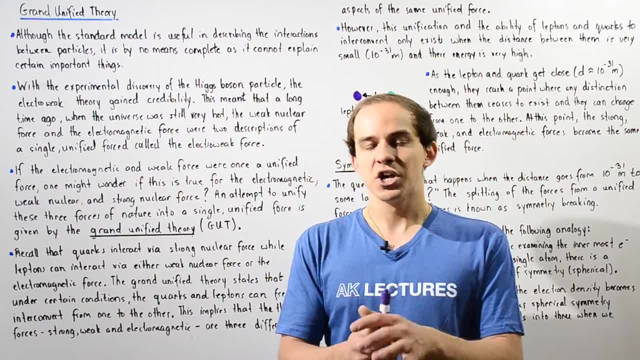 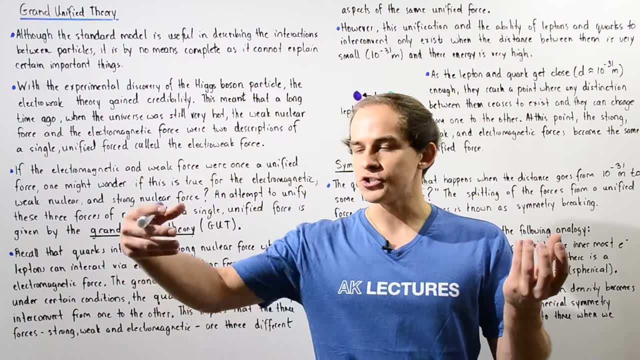 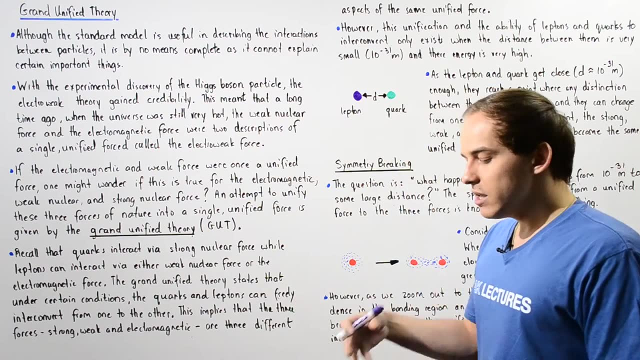 single force known as the electroweak force. can we actually combine the electroweak force, the combination of the electromagnetic and weak nuclear force, into a single force with the strong nuclear force? So can we combine the three forces in nature known as the electromagnetic? 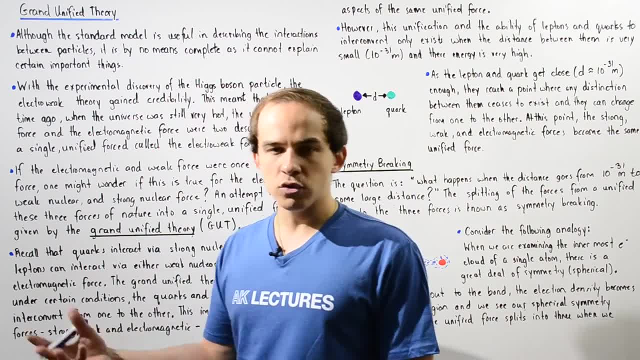 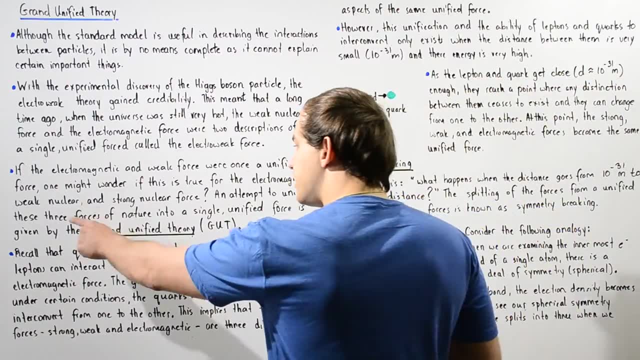 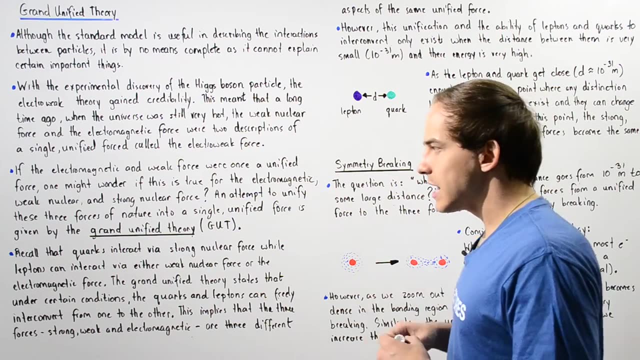 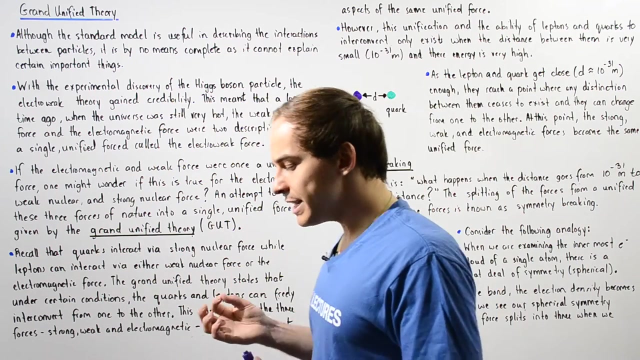 force, the strong nuclear force and the weak nuclear force into a single unified force. Well, an attempt to unify these three forces of nature into a single unified force by theoretical physicists has been made, and this is called the Grand Unified Theory, or GUT. Now the 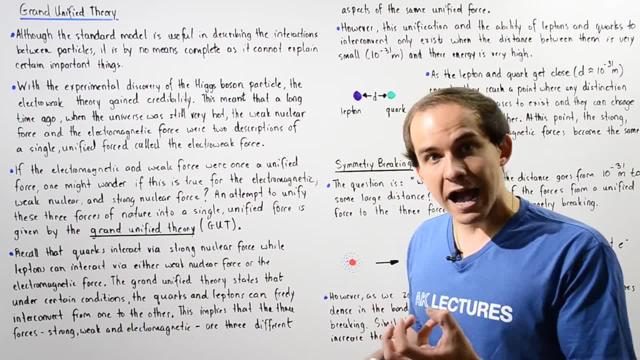 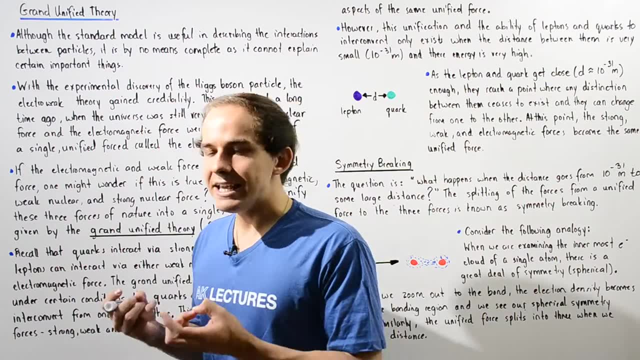 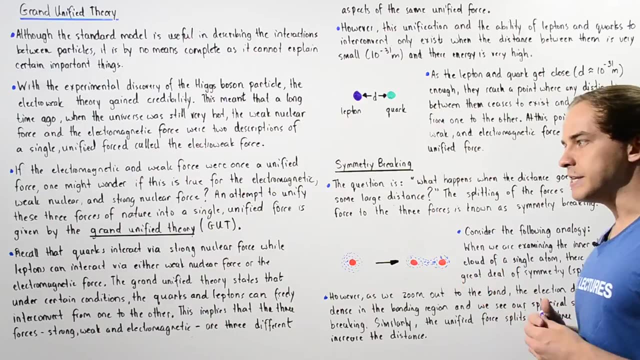 Grand Unified Theory is by no mean a fact. This is basically an idea that has been proposed by theoretical physicists that is being tested Right now, so scientists are basically trying to determine whether or not this is in fact true. So let's recall some information about quarks and leptons. So quarks and leptons. 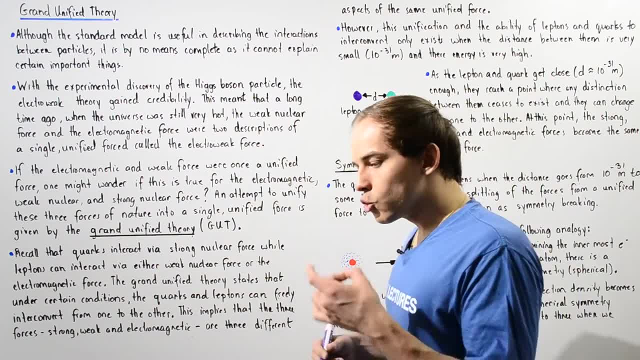 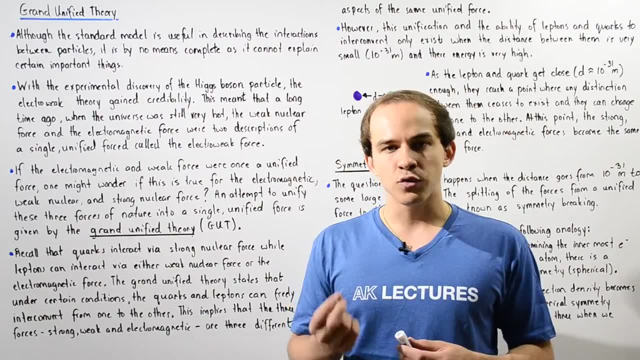 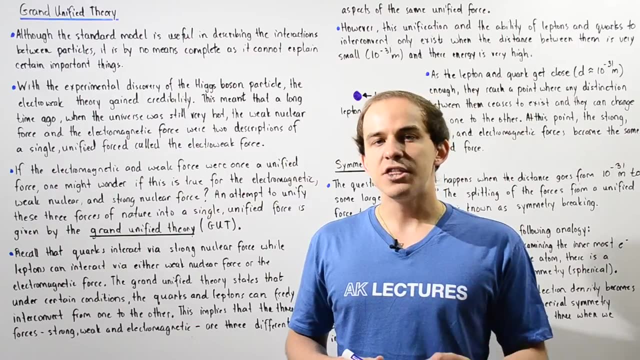 are the fundamental particles in nature, So quarks are those fundamental particles that interact via gluons, that is, they interact via the strong nuclear force. However, leptons are fundamental particles, So quarks are those fundamental particles that do not interact via the strong nuclear. 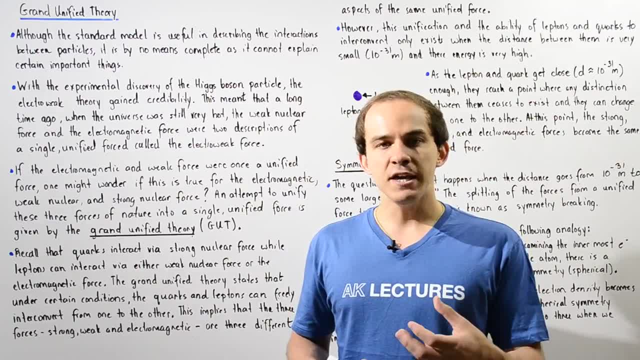 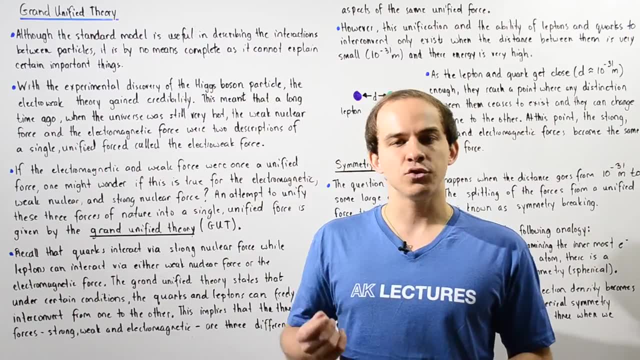 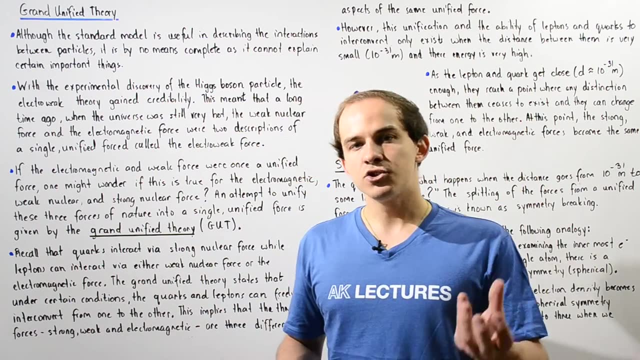 force. They interact predominantly via the weak nuclear force and if they have charge, such as the electron or the muon, they can also interact via the electromagnetic force. So quarks are particles that interact via the strong nuclear force. Leptons are particles. 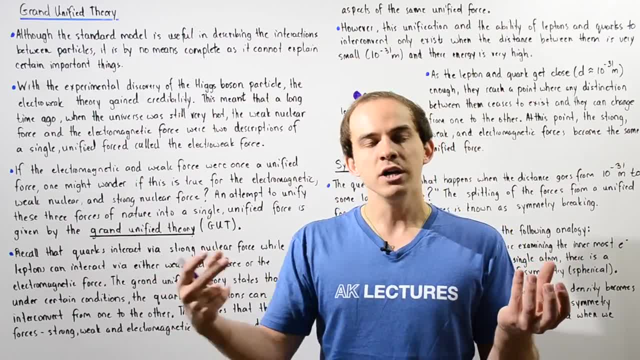 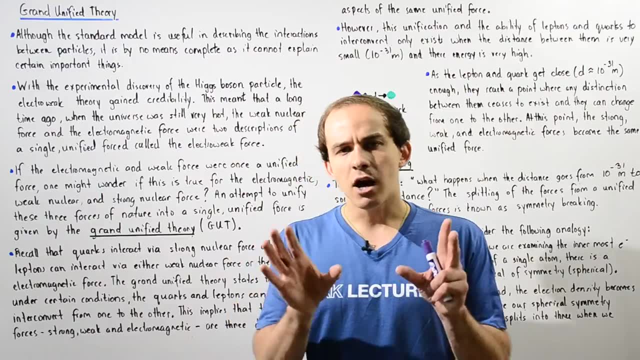 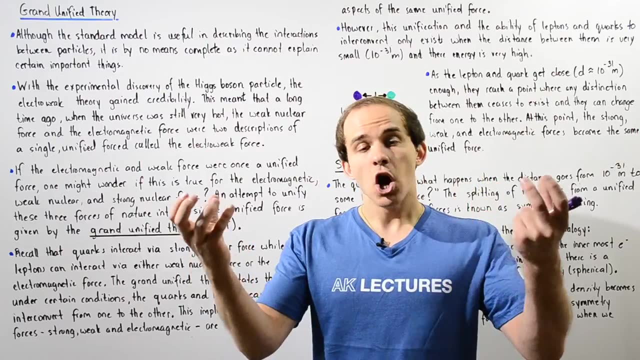 that can interact via the electromagnetic force or the weak nuclear force. Now, what the Grand Unified Theory does is: it states that under certain conditions, when our leptons and when our quarks are very close to one another and their energy is very high, 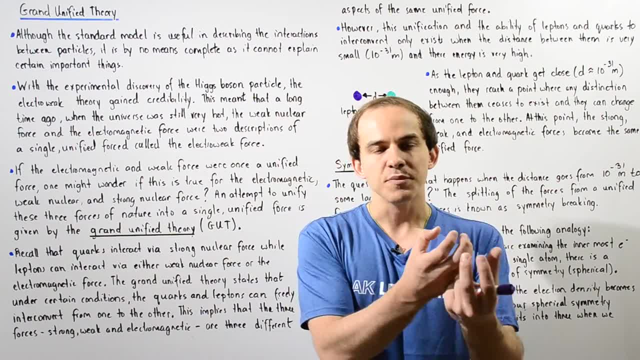 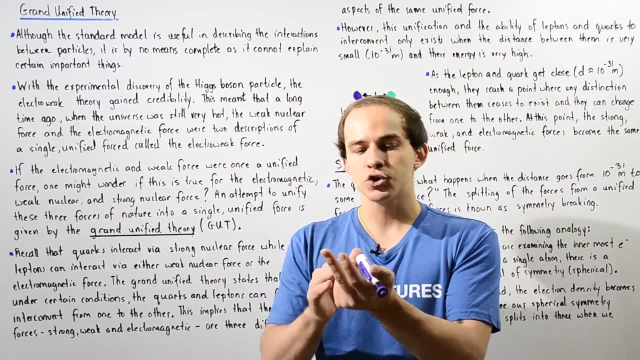 they can basically interconvert from one to the other. And as they interconvert we see that all these three forces- the electromagnetic force, the strong nuclear force and our weak nuclear force- basically interact. So quarks are the fundamental particles that interact. 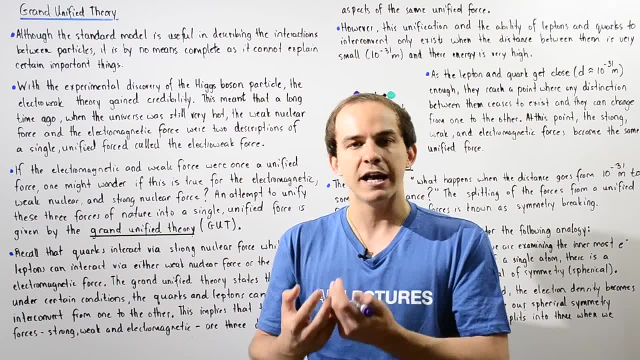 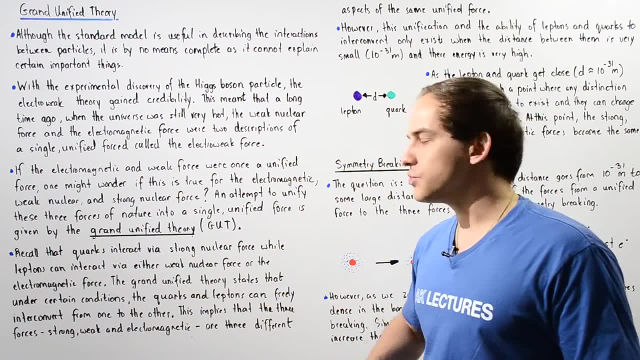 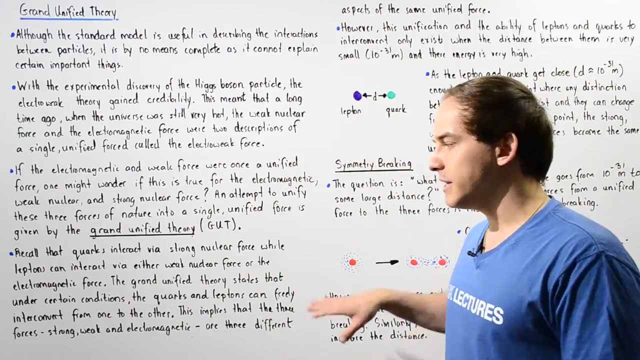 via the strong nuclear force. So once again, the Grand Unified Theory states that under certain conditions, the quarks and leptons can freely interconvert from one to the other, And this basically implies that these three forces in nature, the strong nuclear force, 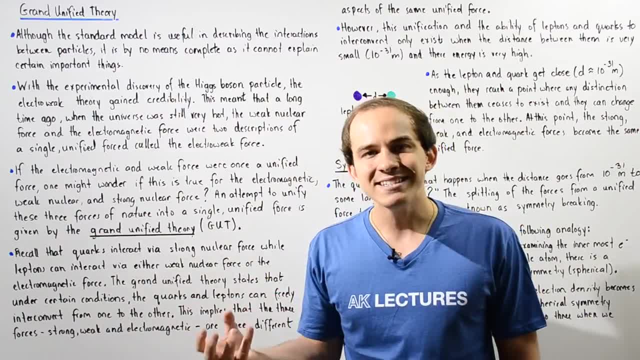 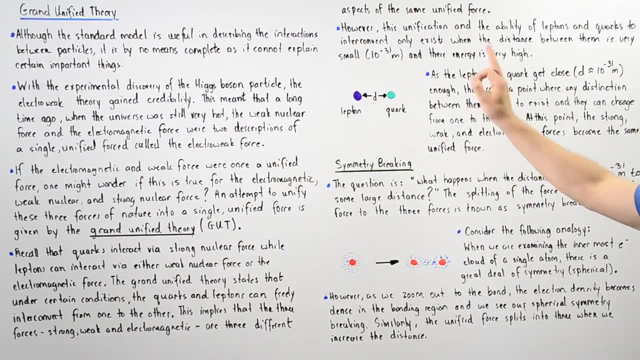 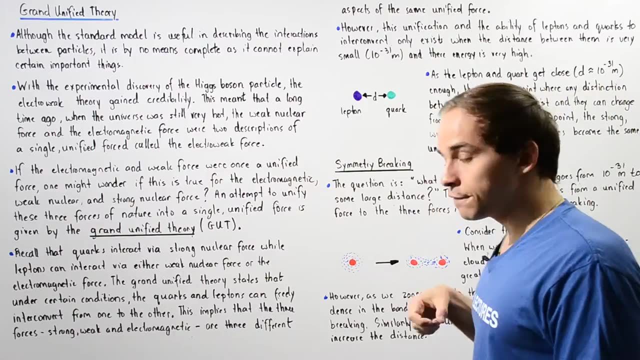 the weak nuclear force and the electromagnetic force are basically different aspects of the same force, The same exact unified force. However, this unification of the three forces and the ability of leptons and quarks to interconvert from one to the other can only be achieved when 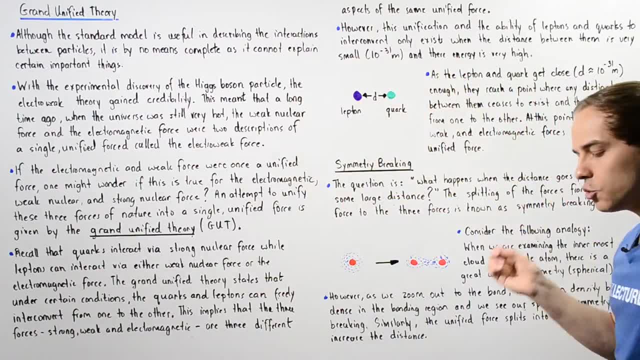 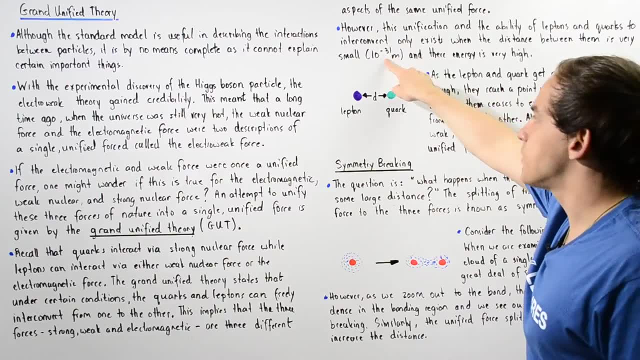 our lepton and quark is found very close to one another when the distance is at least one times ten to negative thirty-one meters. So basically, when they get this close they can interconvert from one to the other. So that's the Grand Unified Theory. 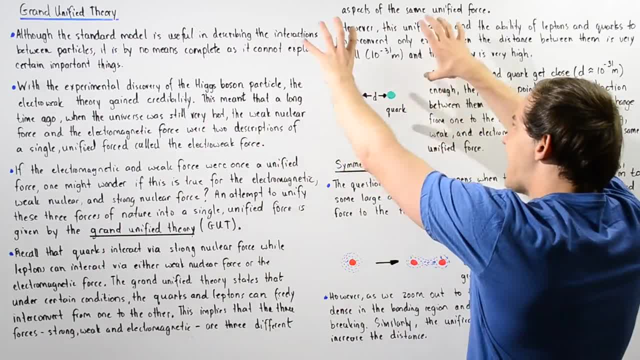 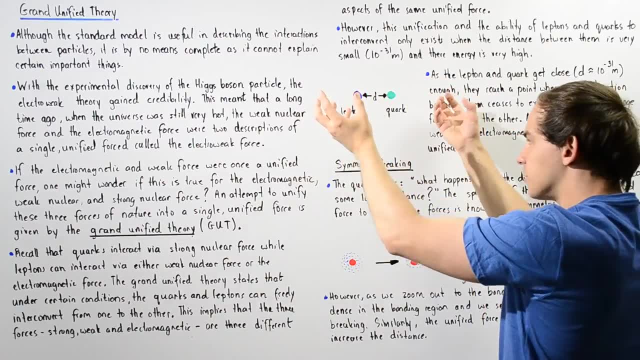 So this is the Grand Unified Theory. So this is the Grand Unified Theory. So when they get this close, the distance is very small and the energy is very high and these leptons and quarks can basically interconvert from one to the other. 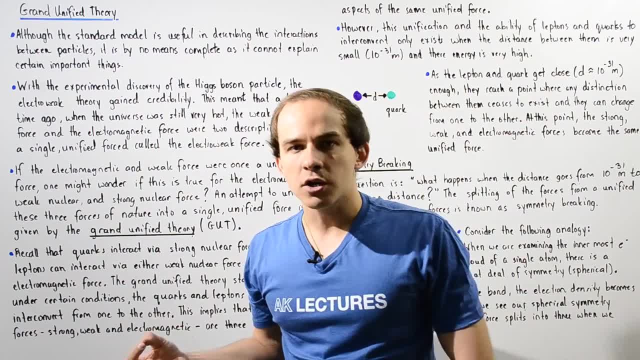 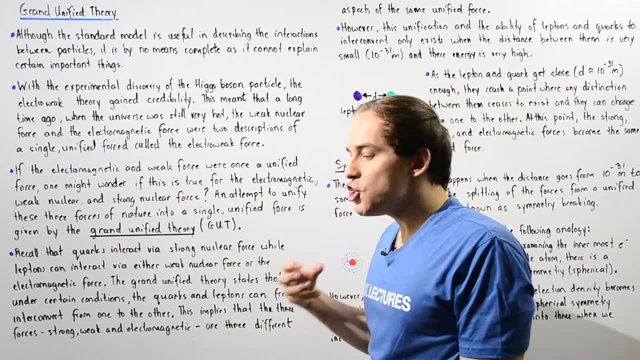 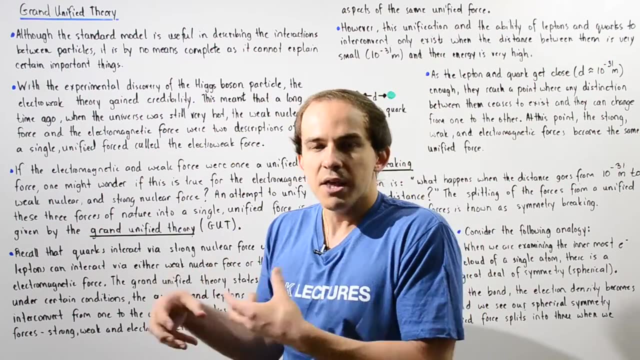 And when they interconvert, there is no longer any distinction between our two particles. That is, we can no longer actually make a clear distinction between our two particles. They essentially become the same type of particles. So this is the Grand Unified Theory. 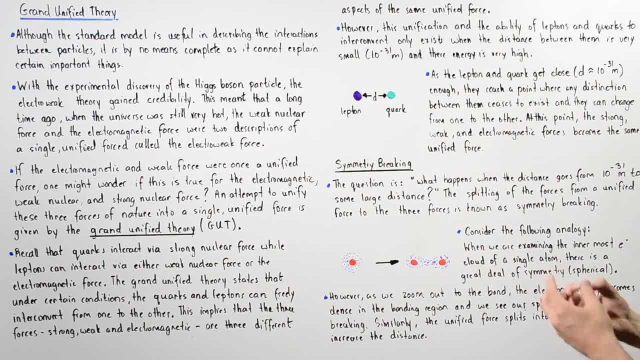 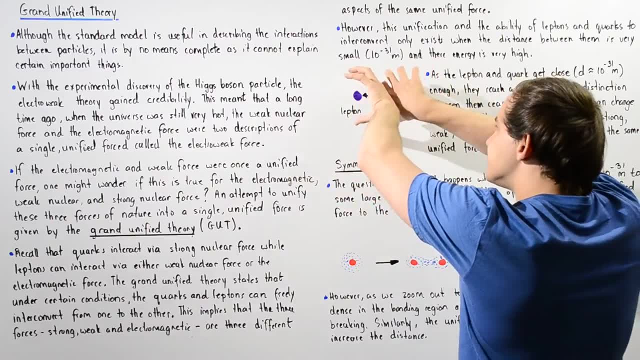 And this is the Grand Unified Theory. So the Grand Unified Theory is to match the same type of particles, and so our three forces unify in to a single unified force. Now, when our particles separate, when the distance is greater than this distance, the 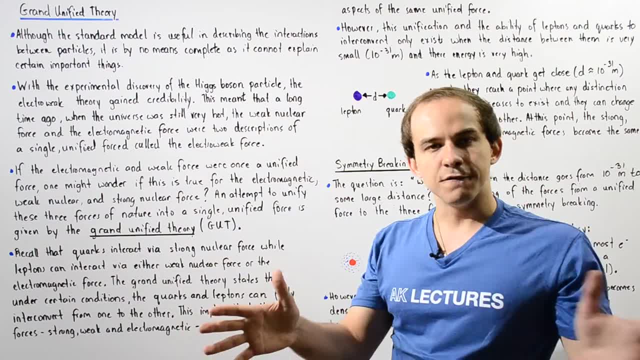 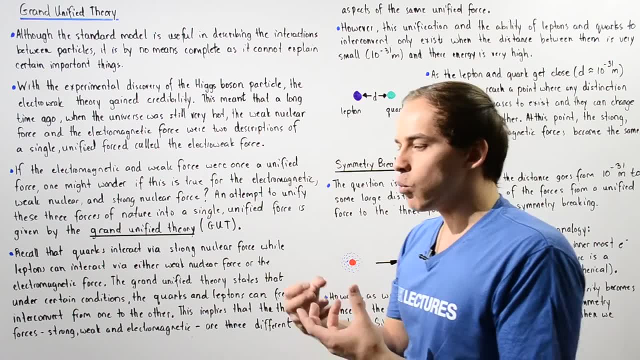 three forces basically split from the unified force to our three different forces, And this splitting point is called Symmetry breaking. So we go from a point where we have a lot of symmetry, where we have an equal distance, then we have a separation point and this separation point is known as Symmetry breaking. 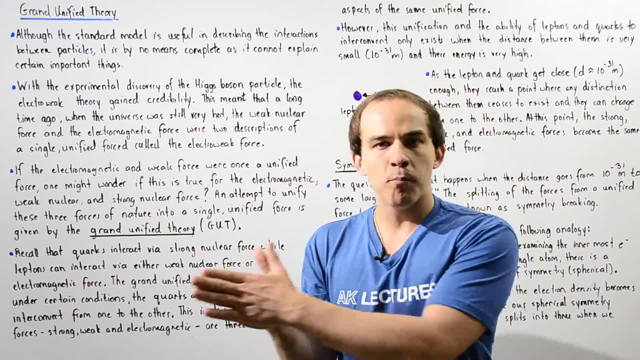 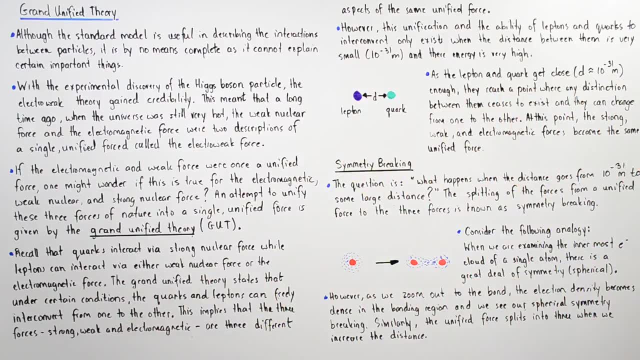 where our forces are unified into a single force to a point when our symmetry breaks into the three different points, the three different forces. So once again, the question is: what happens when the distance goes from this distance, our unification distance, to some large distance? 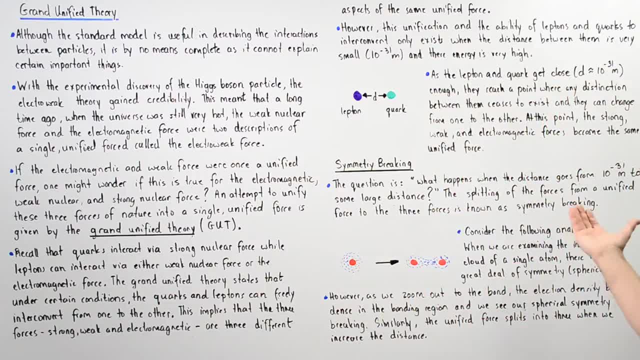 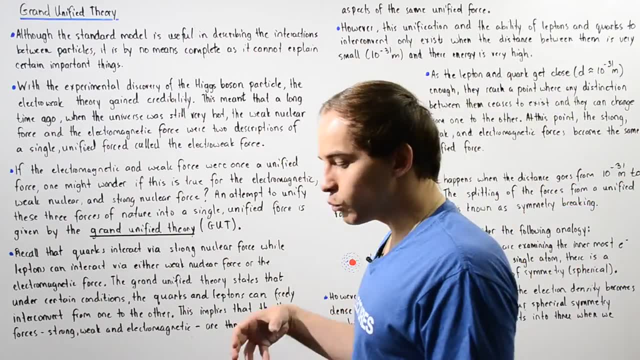 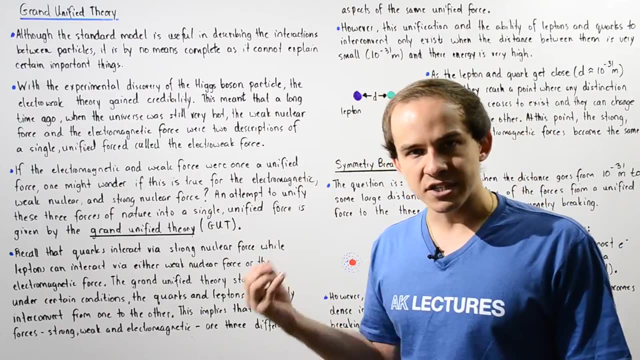 Well, the splitting of this unified force into the three different forces of nature takes place, and this process is known as symmetry breaking. In fact, we spoke about symmetry breaking when we discussed the electroweak theory in the previous lecture. We said that when the electromagnetic force 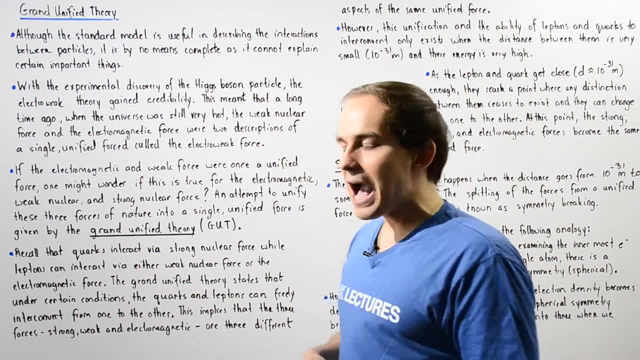 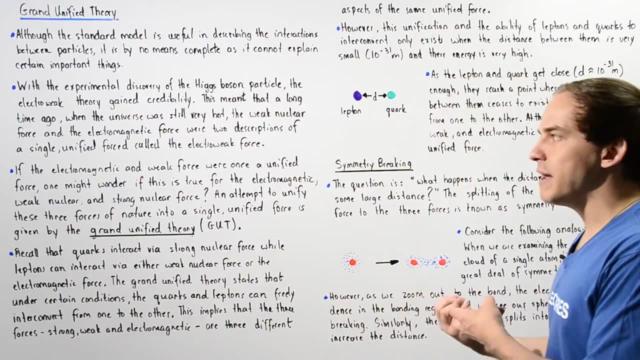 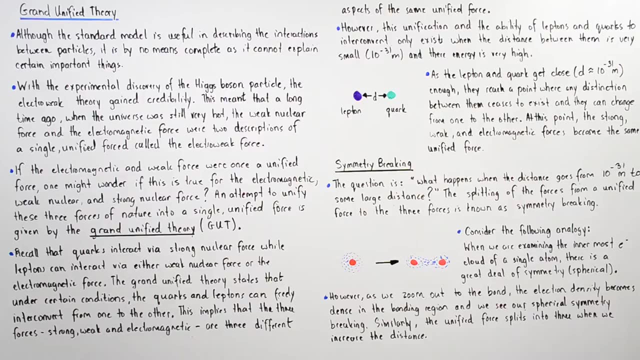 and our weak nuclear force split from our electroweak force. that was known as spontaneous symmetry breaking and that was basically confirmed when we discovered experimentally the Higgs boson particle. Now to understand the concept of symmetry breaking, let's consider the following analogy: 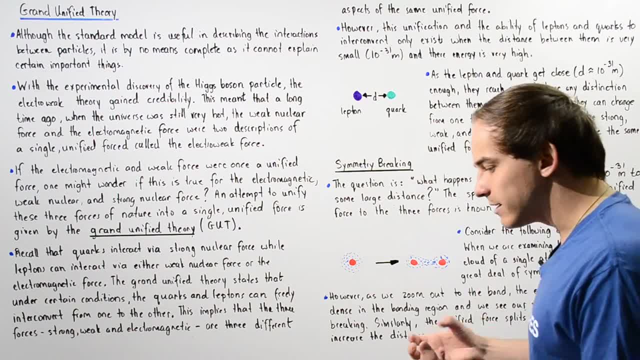 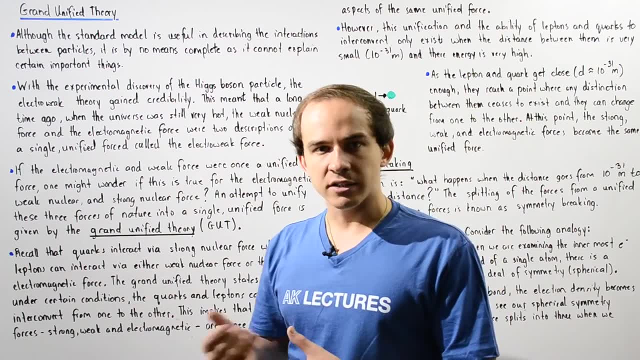 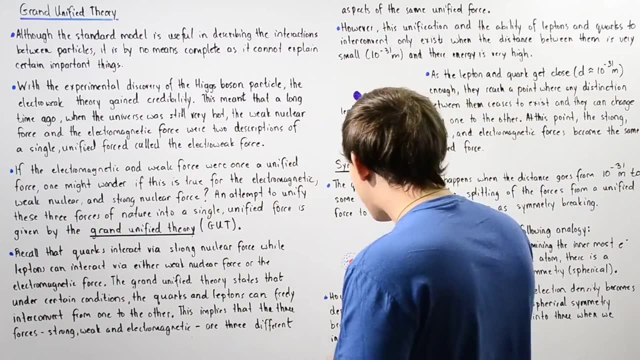 Suppose that we are examining a single atom. So we have a single atom, as shown, and we're looking at the inner electron cloud, at the inner electron density. So, for example, if we take the hydrogen atom, the hydrogen atom has one electron. 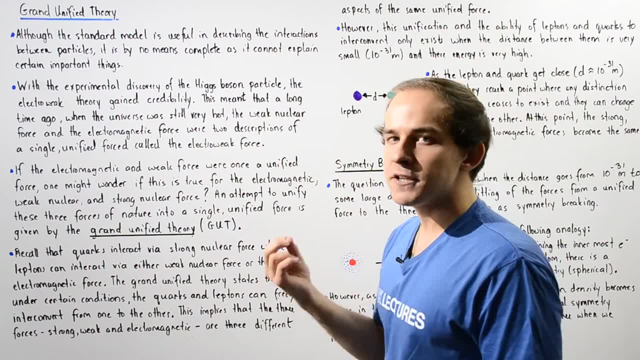 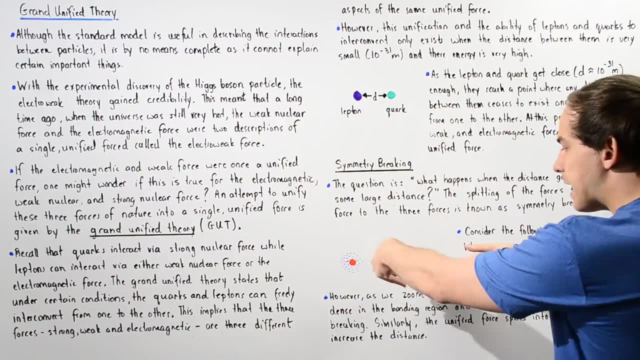 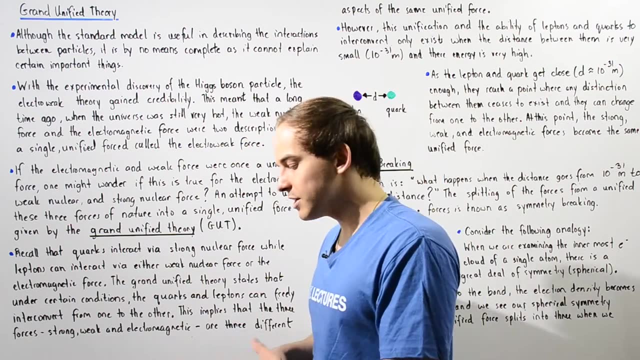 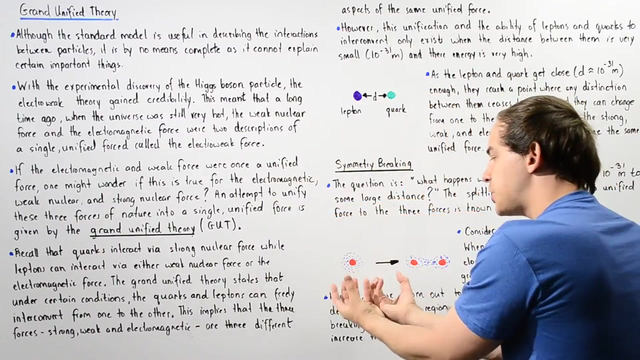 It creates this electron cloud that is perfectly symmetrical. It is perfectly spherical. However, if we zoom out and we examine the chemical bond that is formed between two hydrogen atoms in a diatomic H molecule, we see that there is symmetry breaking. We no longer have this spherical shape. 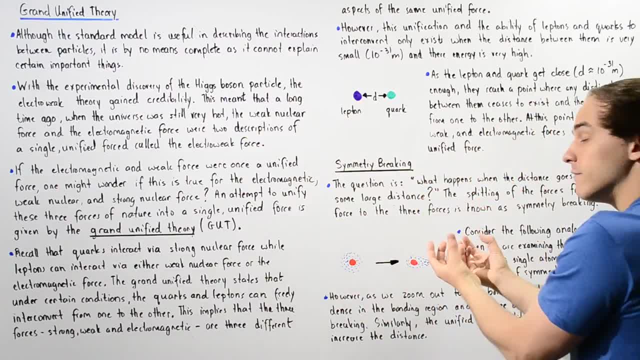 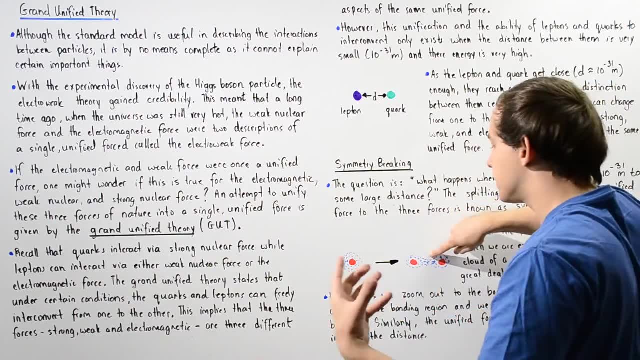 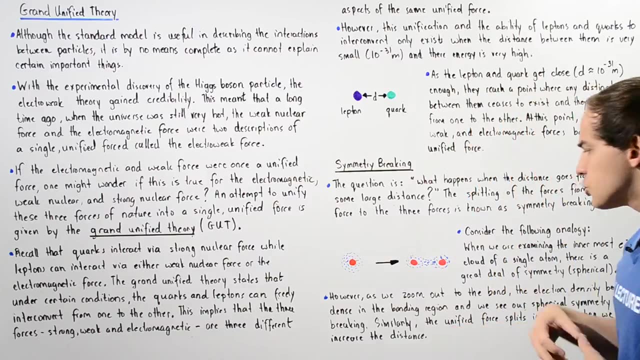 this spherical symmetry. Our density of electrons is now, you know, now found between our two nuclei, within this region we call the chemical bond, And this is known as symmetry breaking. So, in an analogous way, when we go from this very small distance, 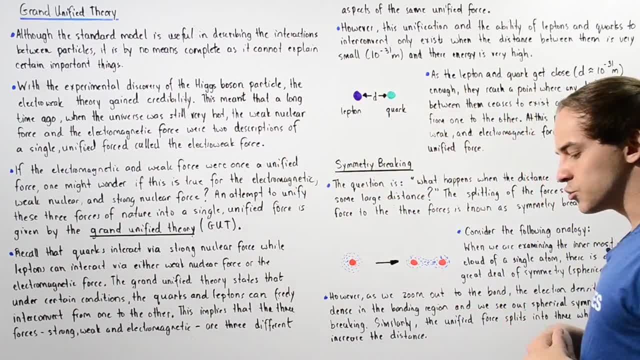 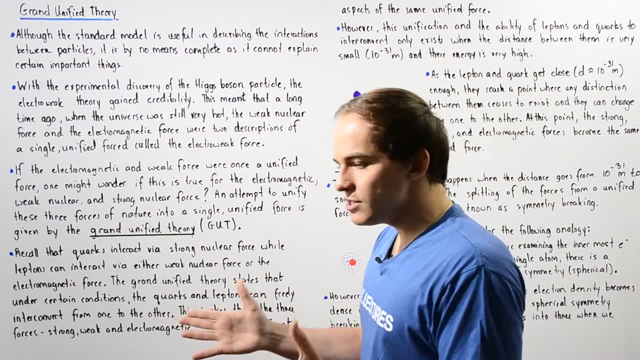 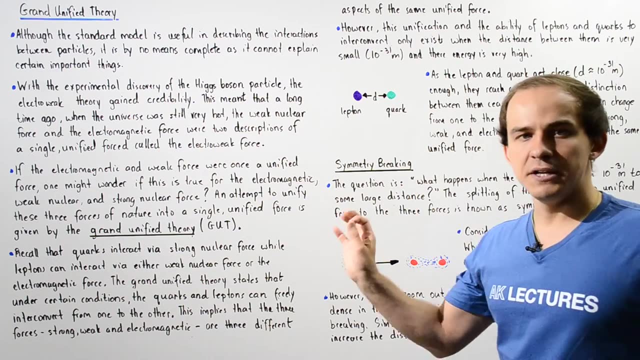 to a distance that is greater than this unification distance, we have symmetry breaking taking place, So our unified force basically breaks into the three different types of forces of nature. So, once again, this has not actually been proven experimentally. This is simply a theory that attempts to explain. 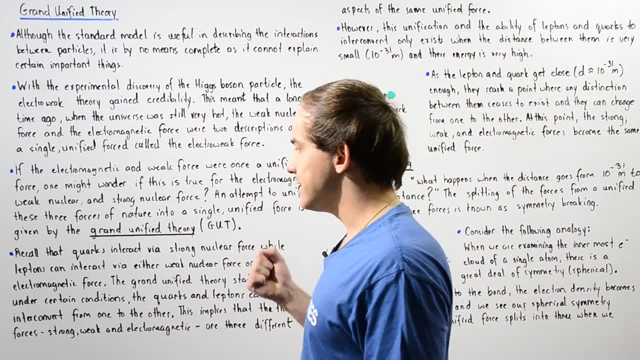 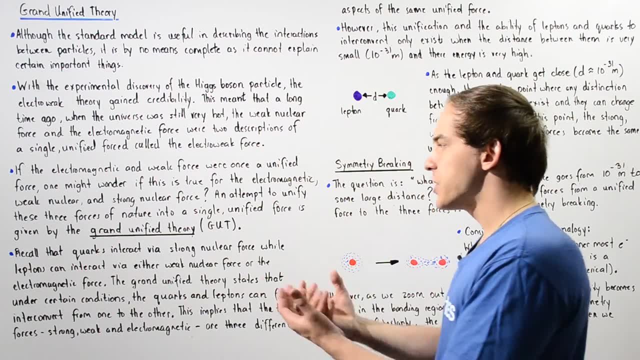 or combine the three different types of forces in nature- electromagnetic force, the weak nuclear force and the strong nuclear force- into a single force, And this theory is known as the grand unified theory.